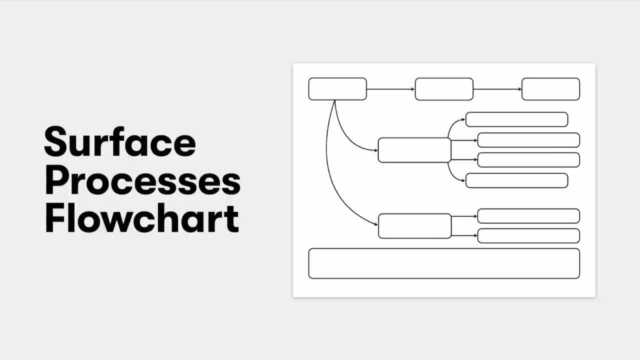 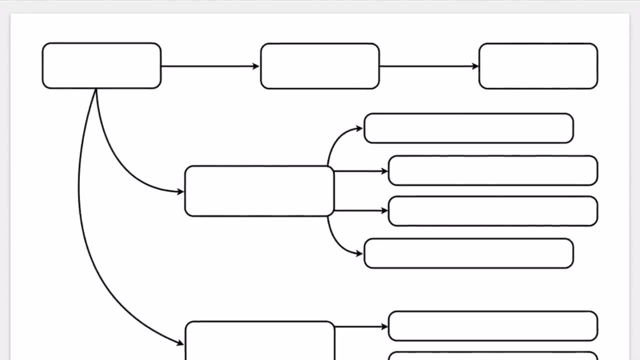 other key ideas. we're going to use this surface process flowchart, which is available on the website, And we'll begin by filling in the three boxes on the top to kind of summarize these three processes, starting with weathering, which we know is breaking apart of rock, and then erosion. 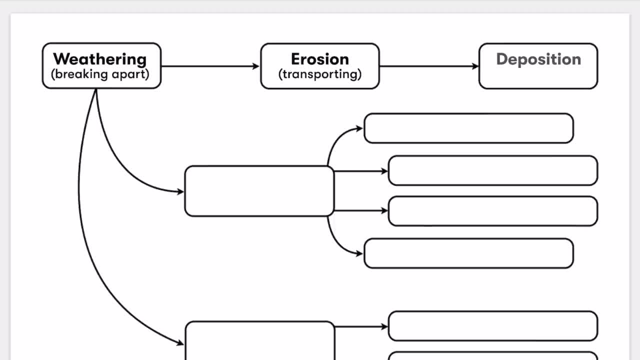 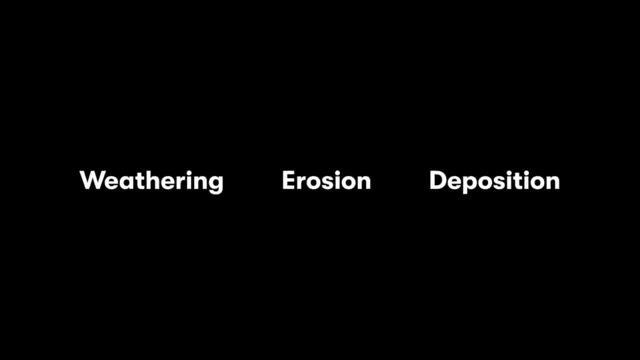 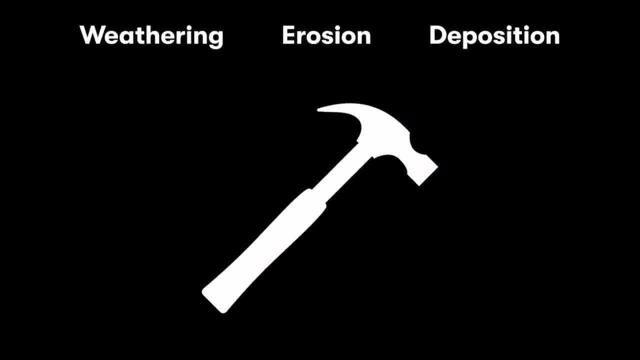 which is the transportation of the sediments, and finally deposition or the dropping off of those sediments. So another way to think about this- this is just kind of a quick analogy that kind of helps me remember the differences between them- is that weathering is kind of like nature's hammer. 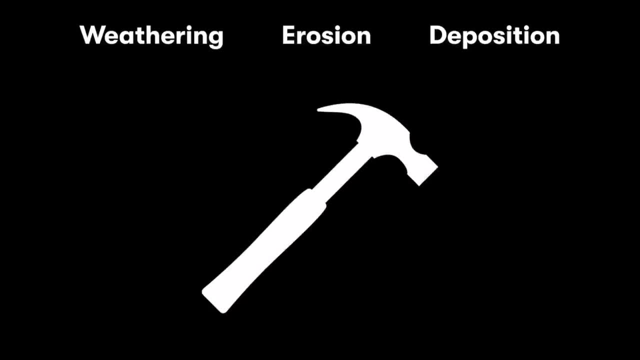 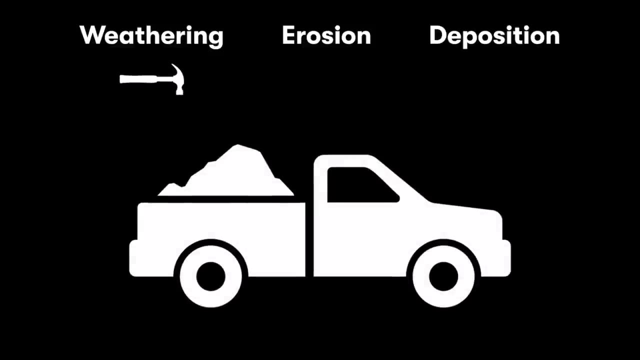 right. It's Mother Nature's way of taking big bits of rock and smashing them into smaller bits or changing them, And then erosion, in this example, would be something like a dump truck or a pickup truck carrying all the little bits and pieces broken apart by weathering, from one location to another. 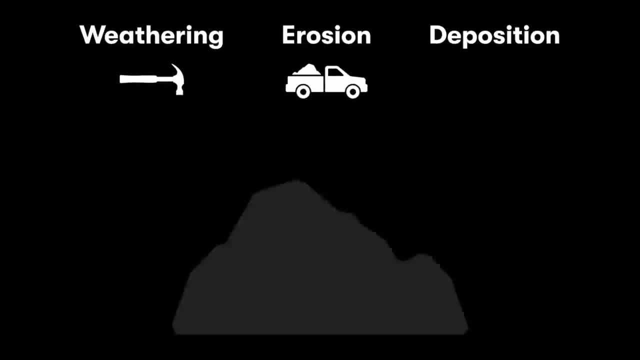 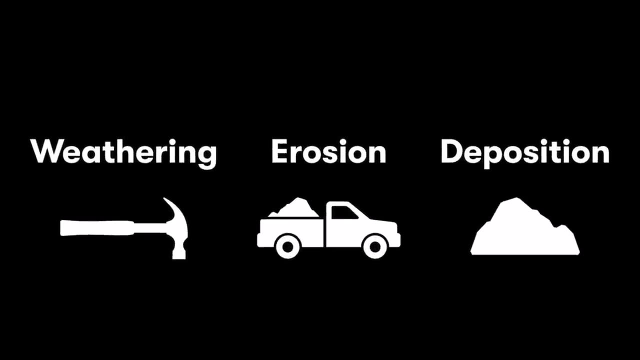 And then deposition is that dump truck kind of opening its tailgate and dumping everything out into a big pile on the ground? That's deposition. So that's just kind of a helpful little way to remember the differences between these three parts of this larger: weathering, erosion, deposition. 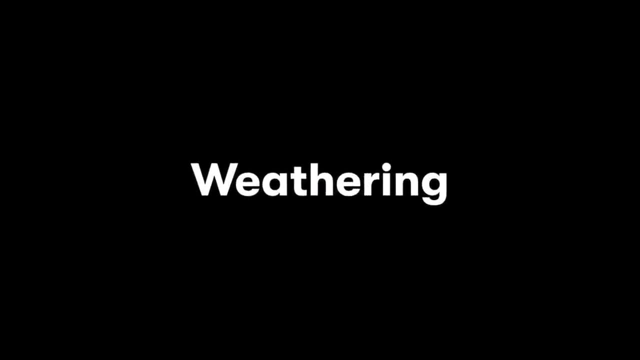 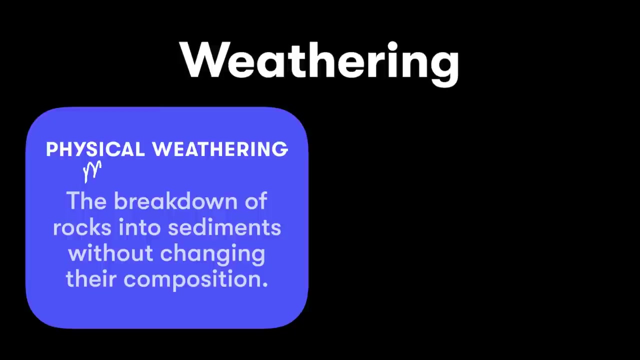 process. Now for the rest of this video. we're really going to focus on weathering specifically, and we're going to start by looking at the two main types of weathering, And the first example we're going to look at is called physical weathering. Now I just want to point out that physical weathering is also often known as mechanical. 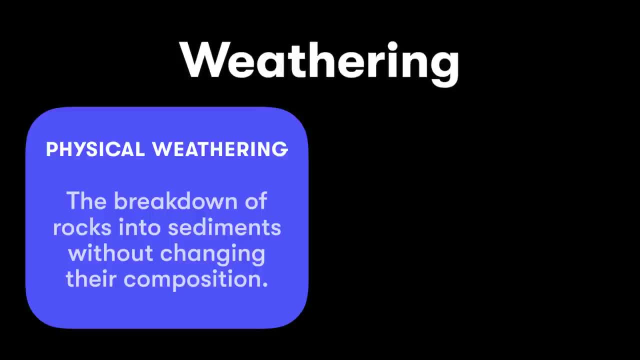 weathering. Okay, so physical and mechanical are the same thing, And this would be the breakdown of rocks into sediments, And the key is that it's without changing their composition. this is literally changing size and shape of a rock. So the waves crashing against a boulder. 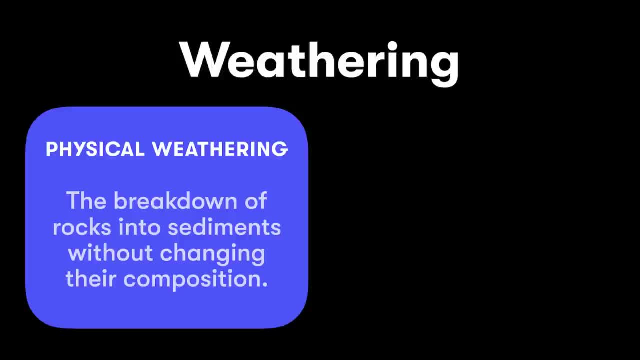 and breaking it into small pebbles. that might be rounded out. That's physical or mechanical weathering, But it's still granite. It's not changing the rock or what it's made of, But that does also happen in nature And we have a different name for that: That's called chemical. 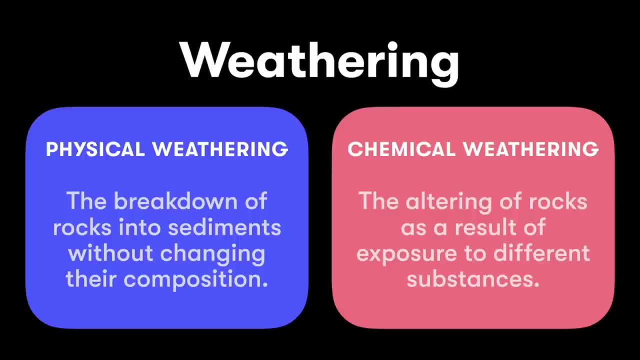 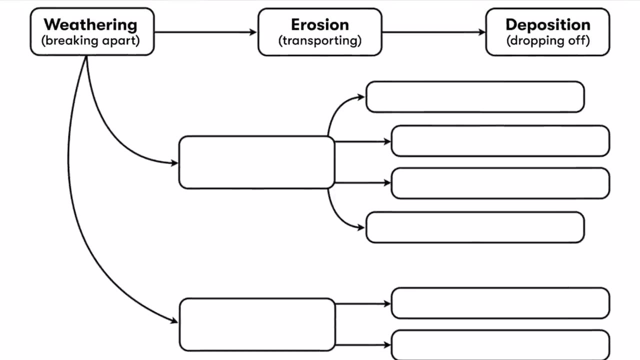 weathering, And so this is when the rocks are changed chemically because of some reaction with usually something like air or water in nature. So the altering of rocks as a result of exposure to different substances. So let's add this information to our flowchart, So we're breaking. 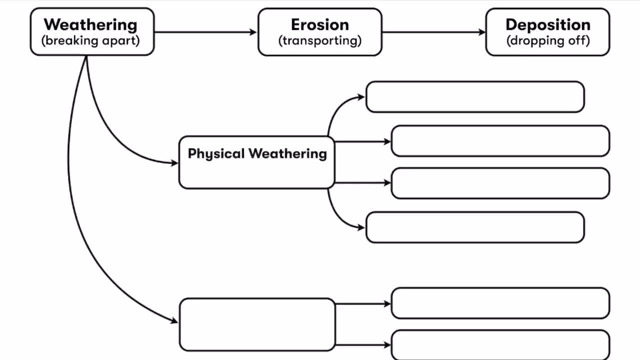 down weathering into two smaller types. The first is physical or mechanical weathering, which is breaking, cracking and grinding, Things like that, And we'll see examples of those shortly. And then chemical weathering, which involves some sort of reaction. 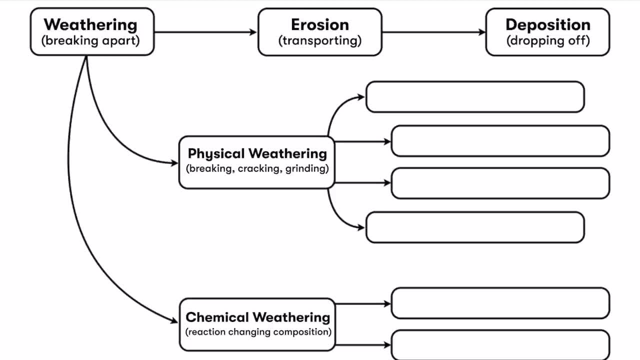 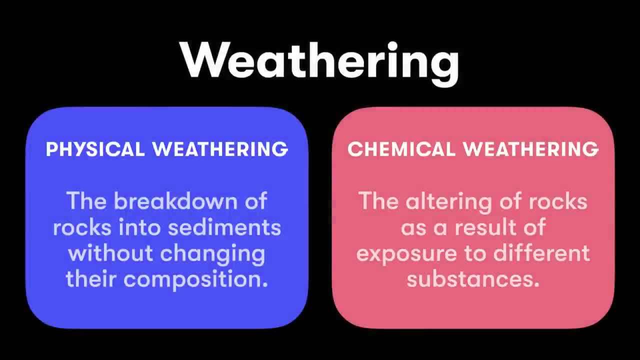 that's going to change the shape of the rock And that's called chemical weathering. That changes composition. So that's a really key difference between the two types of weathering. So let's dive a little deeper into our physical or mechanical weathering and look at some different 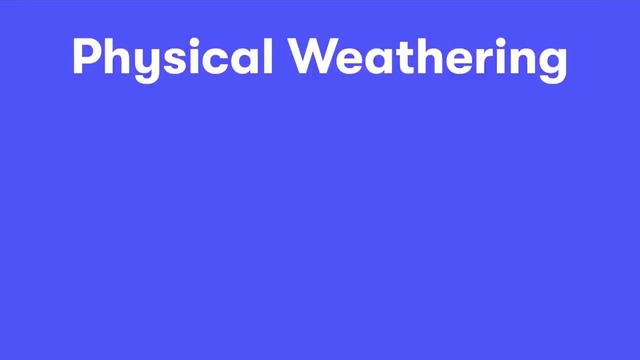 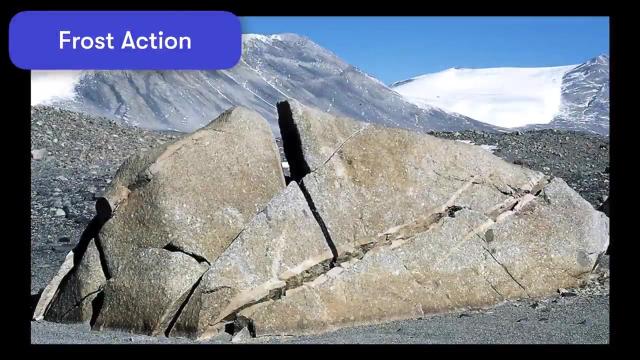 examples. For our purposes, we're going to break this into four specific types: Frost action, exfoliation, abrasion and root wedging. So we will start with frost action, which, by the way, is also known as ice wedging. There are a lot of different names for it. 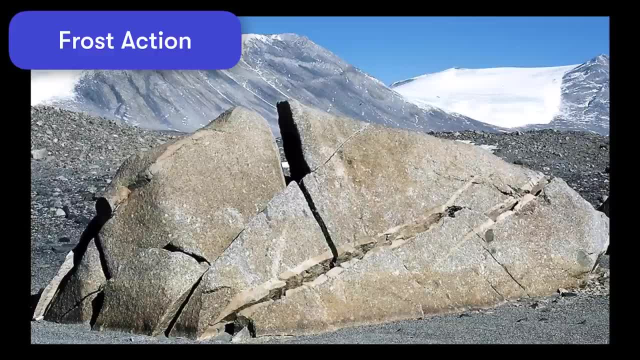 And, as you might imagine, this involves ice, And so what happens is take an area that maybe it's a little bit above freezing temperature during the day and you get some rain, or maybe some melting snow, and you have some water that seeps into the cracks within a rock right, And then the sun sets. 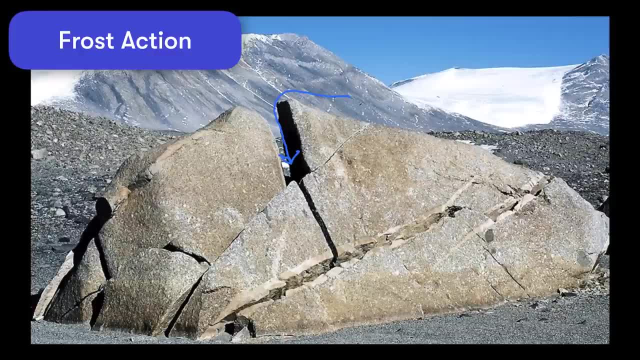 and inevitably the temperature drops and that water freezes into solid ice. Now you may know already, when water freezes, it expands into solid ice, And that's because the water freezes into solid ice. It expands slightly and it gets a little bit bigger. And so, as it expands, it's going to be. 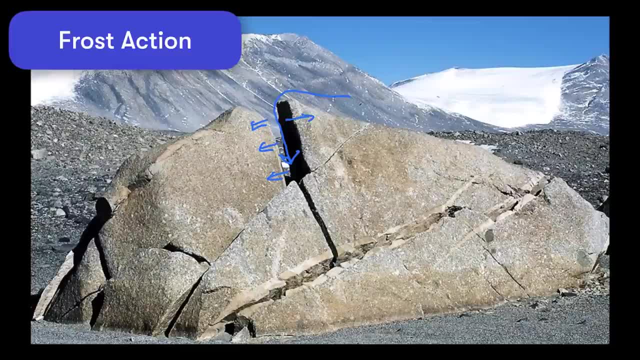 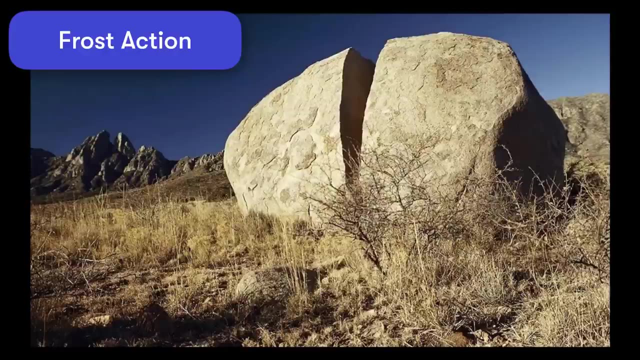 pushing outwards on the rock that it has seeped into, And that force, believe it or not, is actually strong enough to very slowly and gradually break apart rocks, And this process is known as frost action or ice wedging. And so we see examples of this in all sorts of areas where 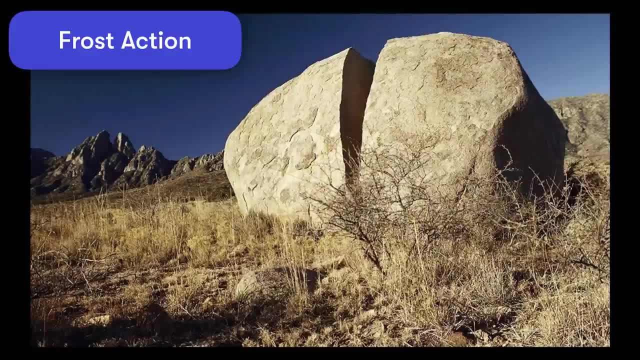 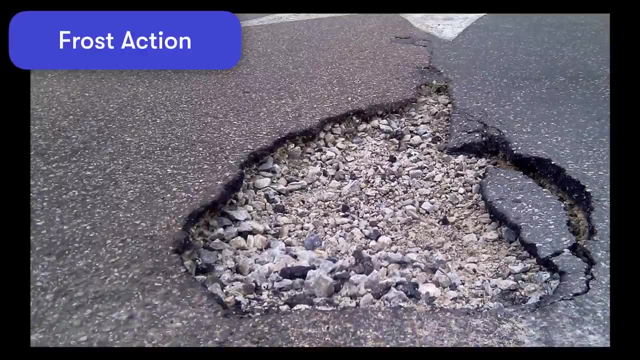 the temperature is a little bit above freezing during the day and then below freezing at night. In fact, a good example of this is what we call a pothole, which you see all over the streets, particularly in the northeastern United States in the springtime, When you have these big fluctuations. 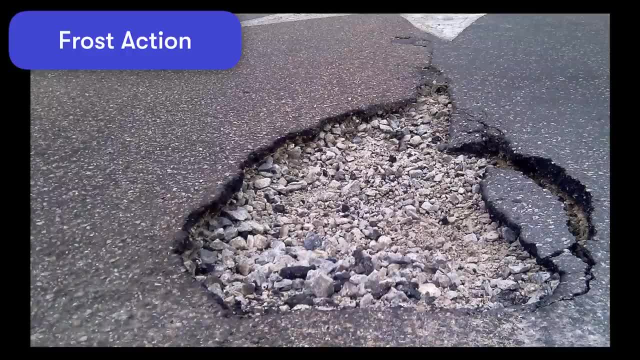 in temperature. the water actually gets into cracks in the road and then freezes and expands And then you drive over it the next day and it just breaks apart and you end up with these big nasty holes in the ground. That's a good example of frost action or ice wedging. Second would be: 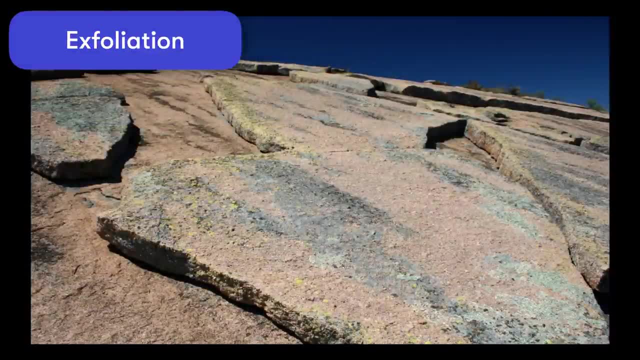 exfoliation, And this is in a way, kind of similar. This involves temperature changes as well. So this occurs in areas where you have really dramatic temperature changes, where it gets very hot during the day and then very cold at night. The, the rock itself, will actually expand slightly in the heat and then contract in the cold. 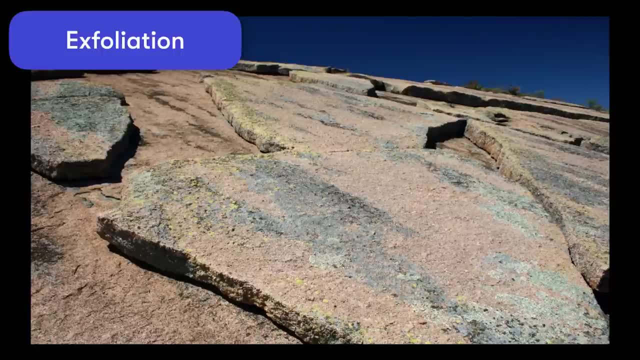 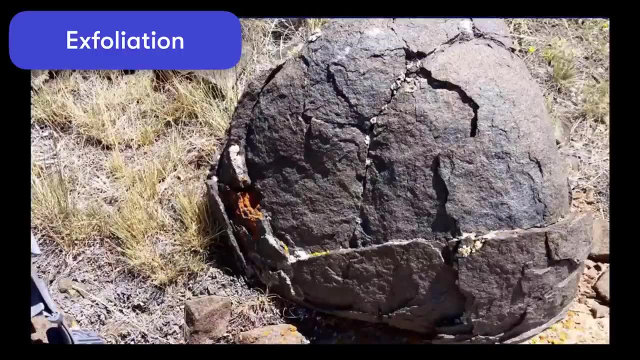 And if this happens day after day, night after night, it weakens the outer layers of the rock until they eventually begin to crack and peel apart like this or like this right here, It's almost like the rock is shedding its outer layer. It's almost like it's breaking into layers and physically or mechanically breaking apart, largely as a result of these. 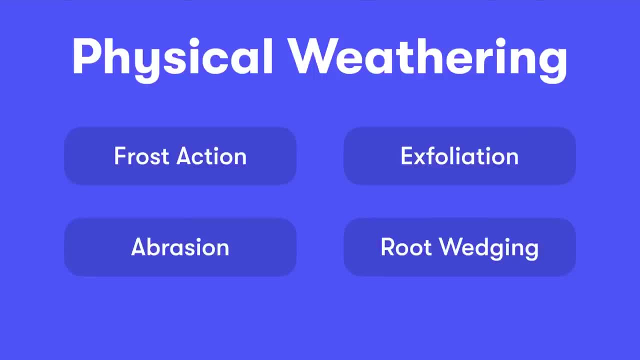 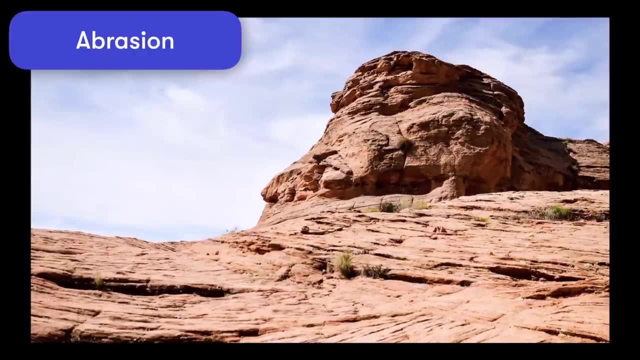 temperature changes. Third example, which is the most common and we see it all over the world, is called abrasion. So abrasion is basically whenever rock grinds against other rock And it comes in many forms, Like here in the desert we see a lot of wind abrasion where 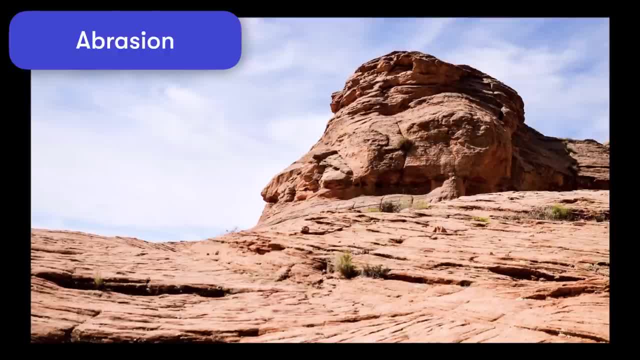 gusts of wind will blow grains of sand that crash into other rock, And very, very slowly, over thousands and thousands of years, we'll actually eat away at the rock, And so wind abrasion is actually responsible for a lot of the interesting kind of rock formations that we see in the American Southwest. 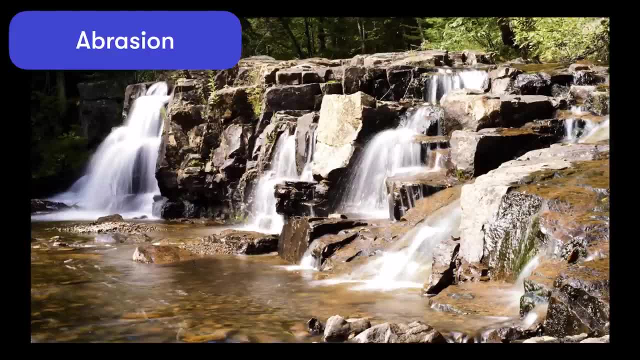 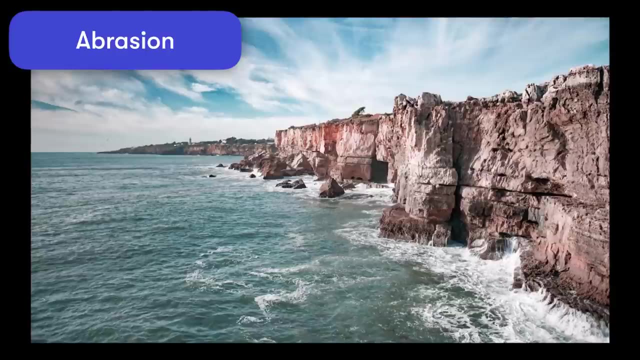 We also can have water or stream abrasion, as little pebbles and sediments are bounced along the bottom of a stream as the water flows And that's going to eat away at the rock that they're bouncing over. We also see this on coastlines, as I mentioned before, with waves crashing into rock and grinding it down by carrying little bits of water. 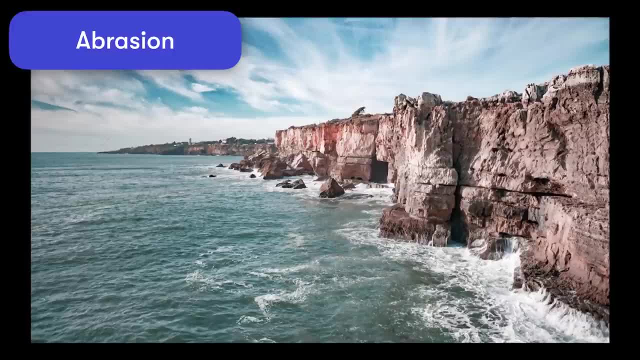 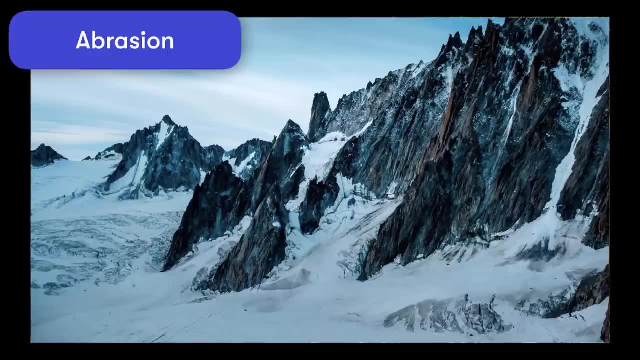 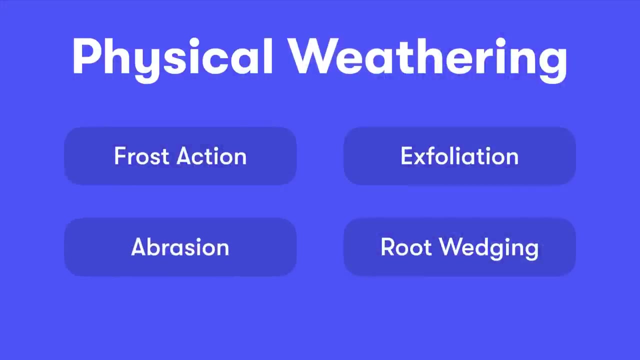 Little bits of sand and sediment and eating away at the rock. And then, finally, with glaciers, Glacial abrasion is very common. Glaciers glide downhill, pulled by gravity, and they scrape along the rock and carve it away over many hundreds of years. Finally, the last type of physical or 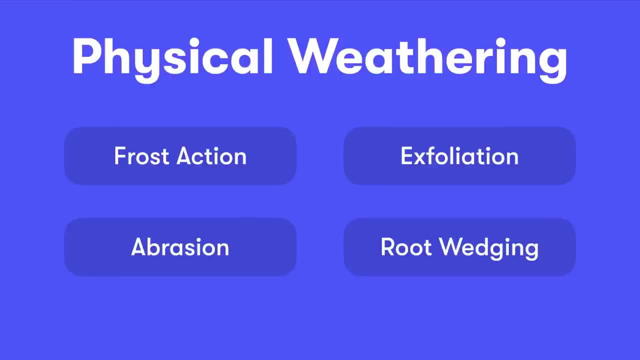 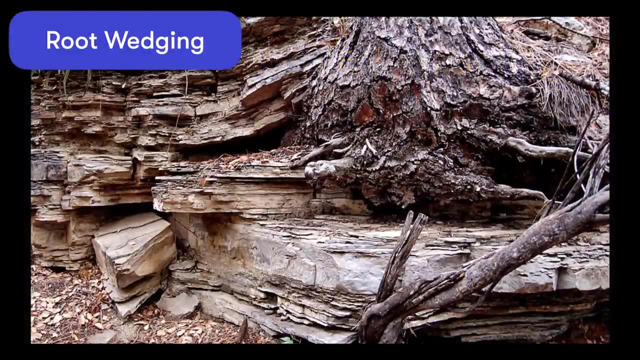 mechanical weathering we're going to look at is called root wedging, And it's pretty self-explanatory. This is when plant roots actually grow within the cracks of rock And as the plants grow larger and larger, they break apart the rock as they grow into it. So we see examples of this. 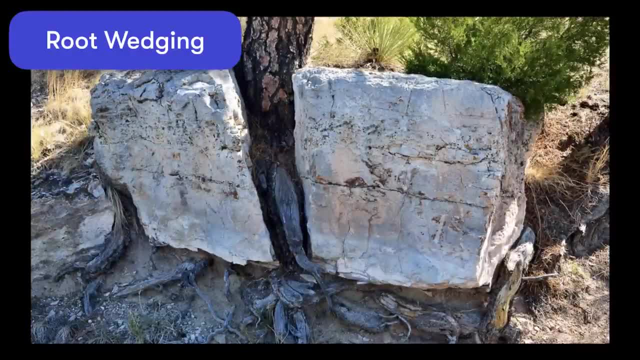 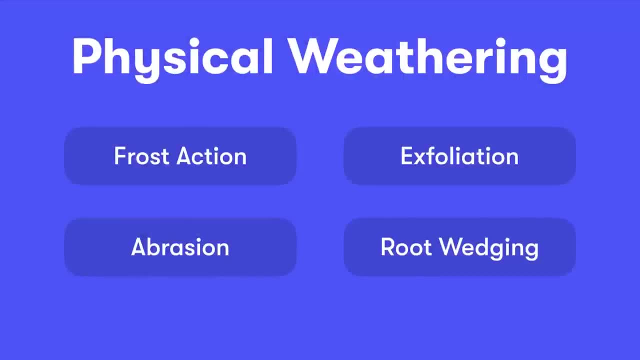 all over the world. It's amazing how powerful tree roots and plant roots can actually be, so much so that they will physically break apart rocks as the plants grow. So those are four main examples of physical weathering, And we want to add them to our flow chart here. So, under our physical 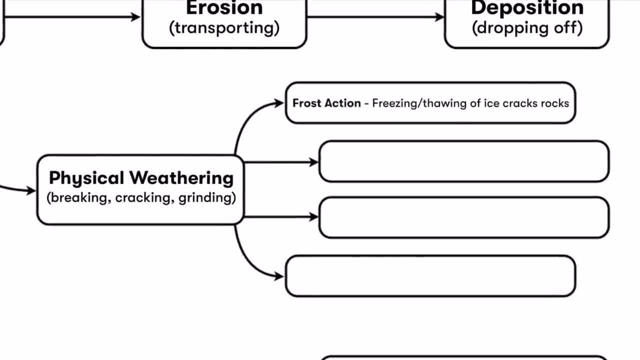 weathering area. we're going to add frost action which is freezing and thawing of ice. It's going to crack apart rocks. And then we're going to add frost action which is freezing and thawing of ice. And then we're going to add frost action which is freezing and thawing of ice. We have 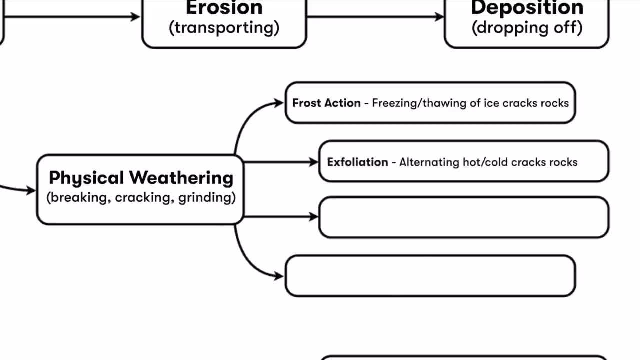 exfoliation, which is the alternating hot and cold, is going to crack rocks. We have abrasion, which is grinding of one rock against another or sand against rock, And then finally, root wedging, which would be our plant roots growing into the rocks. And so those are our four main. 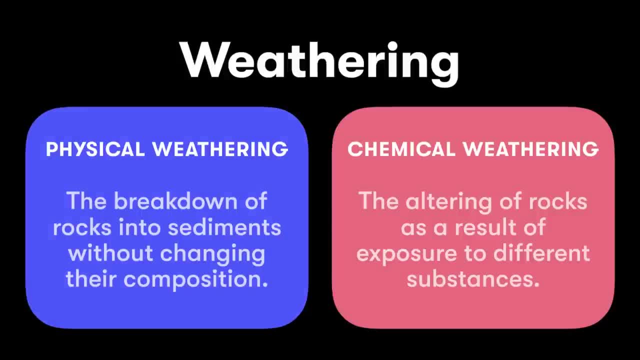 types of physical weathering. Now let's shift gears and look at the second type of weathering: chemical weathering. So remember, this is the altering or the changing of rock as a result of temperature to different substances, And we're going to look at two main examples of this. 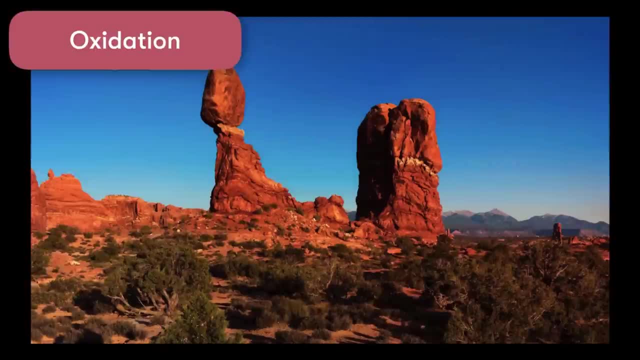 oxidation and carbonation. We'll begin with oxidation, which is a term you may have heard before. It's the formation of rust, And this is going to occur whenever the element iron is exposed to oxygen, And that can happen in the air or in the water. And so what we find are that there. 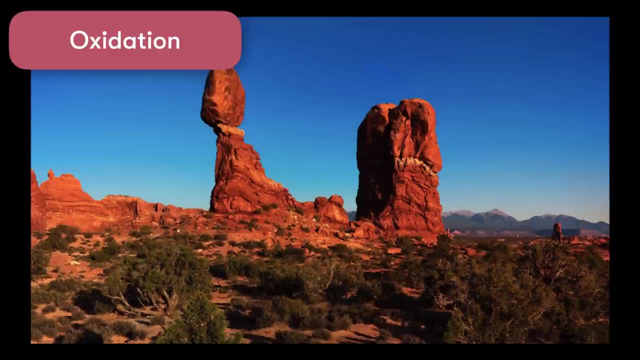 are a lot of rocks around the world that contain large amounts of iron, And as that iron reacts with the oxygen in air or water, it can cause a very serious weathering, And this happens in the. it's going to physically rust And the result is that we see rocks that look like they've been. 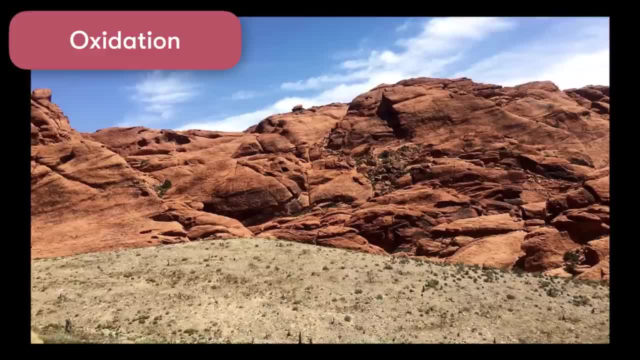 rusted. They have this orangey color to them And that is actually a form of chemical weathering. This rock is breaking down. The rust is very crumbly, this iron oxide that forms and it breaks apart the rock over time. It's an actual chemical reaction with oxygen in the air or the. 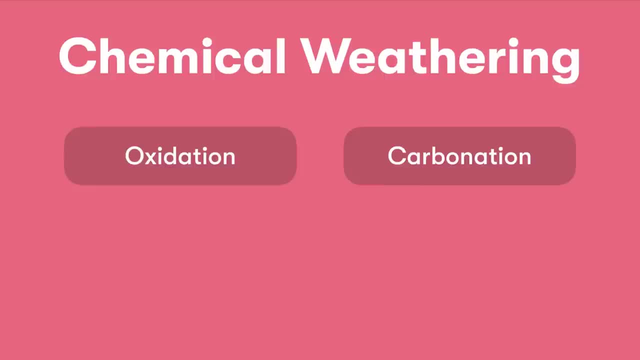 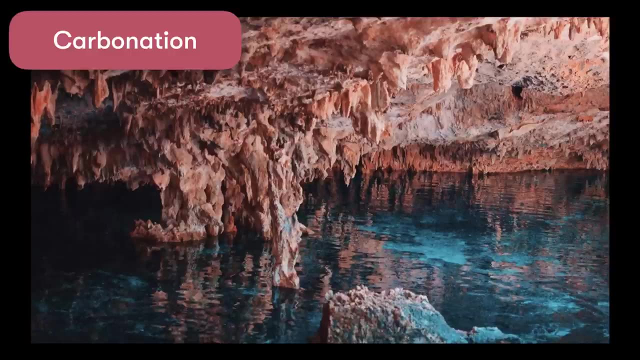 water, And then, finally, we have carbonation. Carbonation is really interesting. This is responsible for the formation of these fascinating, beautiful limestone caves that we see around the world, And it's basically when water flows through the ground it reacts with the different 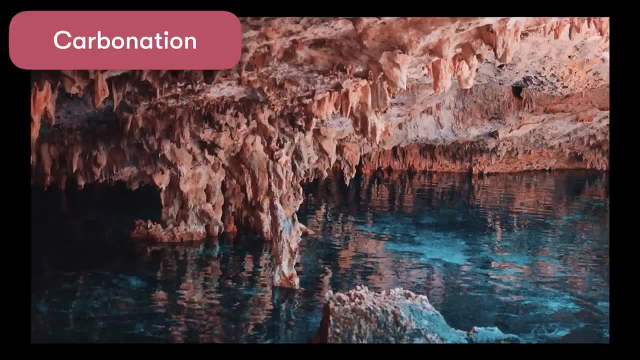 materials in the soil to create a very mild acid, this carbonic acid. And carbonic acid is strong enough that if it encounters certain minerals or rocks like calcite or limestone, it will eat away or dissolve that limestone. And that's what we're looking for. And that's what we're looking for. 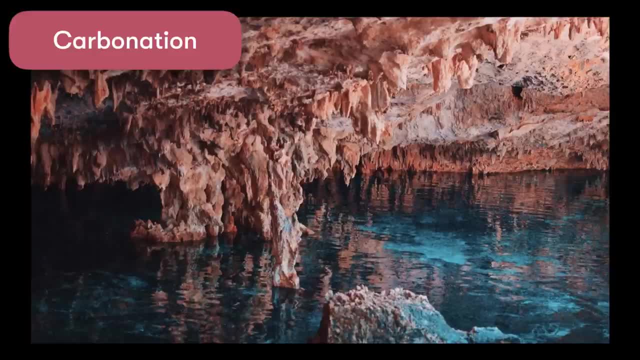 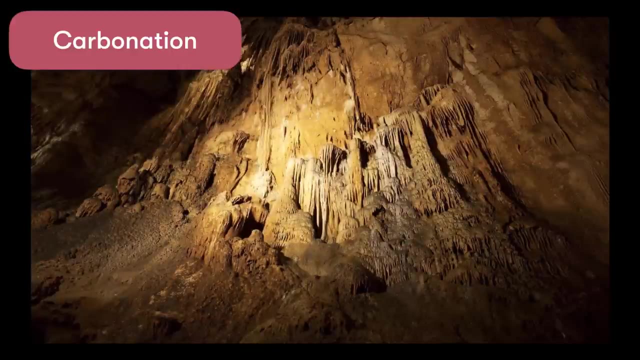 And so what we end up getting are these underground caverns where there once was a whole large expanse of limestone, but that has all been kind of eaten away slowly by the dissolving of this carbonic acid. So we see some of these amazing, amazing landscapes around the world formed as a 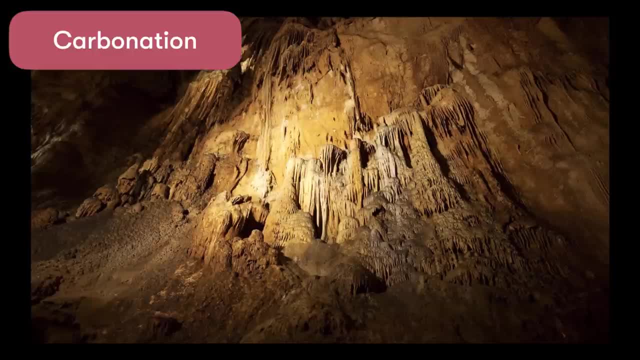 result of this type of chemical weathering. Another thing that happens with this carbonation is that sometimes the ground will actually give way, because all the rock beneath it has been eaten away. And that's what we're looking for, And that's what we're looking for, And that's what we're looking for. 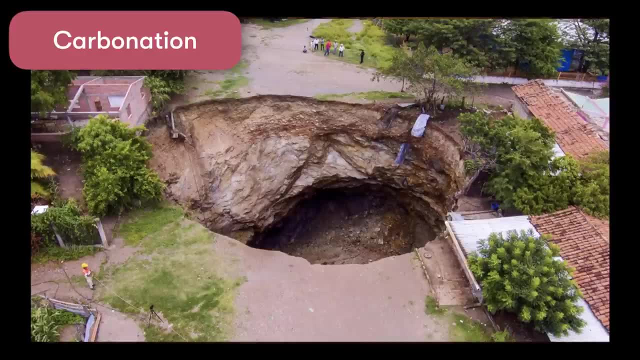 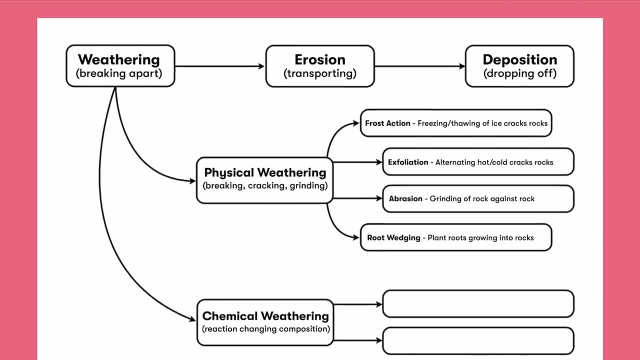 It's when we get something like this, which is called a sinkhole, which is when the rock is gone beneath and the ground collapses above. And so those are two types of chemical weathering, And again we'll summarize them on our flow chart. So the first type was oxidation, Iron and oxygen. 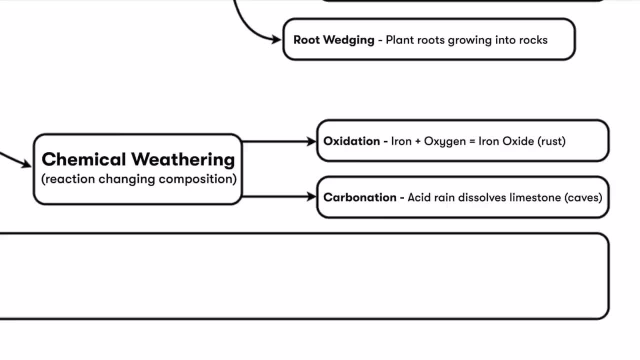 gives you iron oxide or rust. And then carbonation, which is when we have this acidic rain and acidic water dissolving limestone and giving us caves. Okay, Now, there are two main types of carbonation. There are two main types of weathering, with some examples of each. We have them nicely summarized. 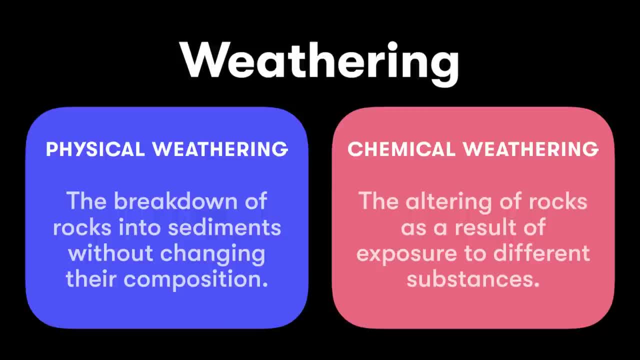 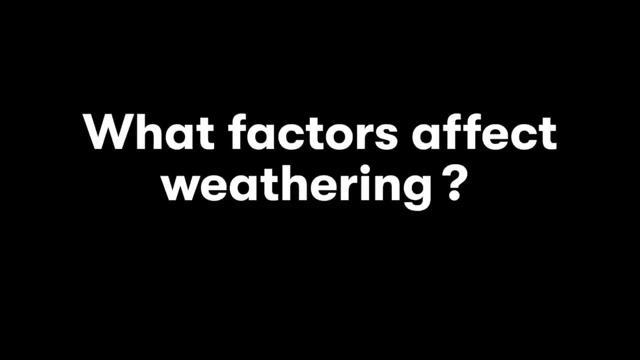 on our flow chart, And the last question we want to ask here is: so what's going to affect weathering, Like, what dictates the type of weathering we have in a region, how fast it will happen, et cetera? And so we have three main things that we're going to look at, And the first: 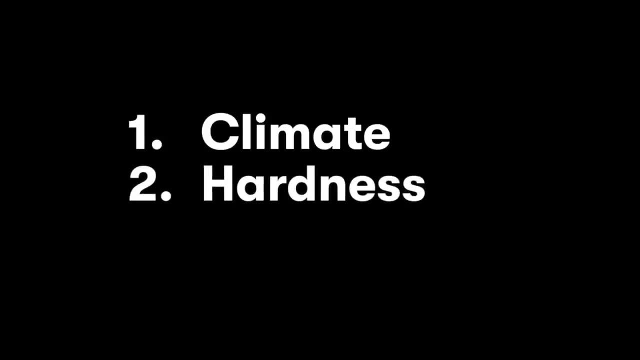 is climate. The second would be hardness: How hard is the rock, or how resistant is it to being weathered? And then the third would be the surface area of the rock. How much of the rock is it exposed to the elements? All right, So let's start with climate, And to understand this, we look at 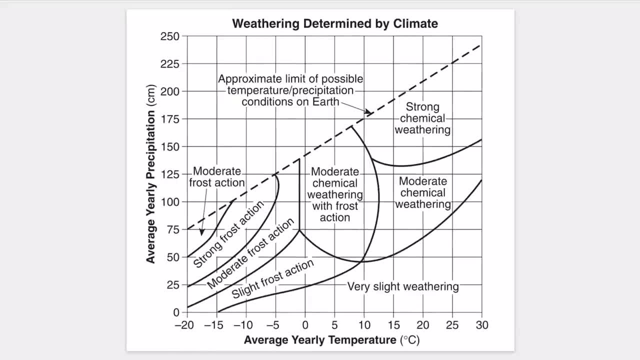 this chart. This is a very commonly used chart in geology, And so what this shows is the effect of the temperature and moisture on what type of weathering will take place. So, for example, in an area that is more hot. so this part of our graph right here which is a higher temperature, okay. 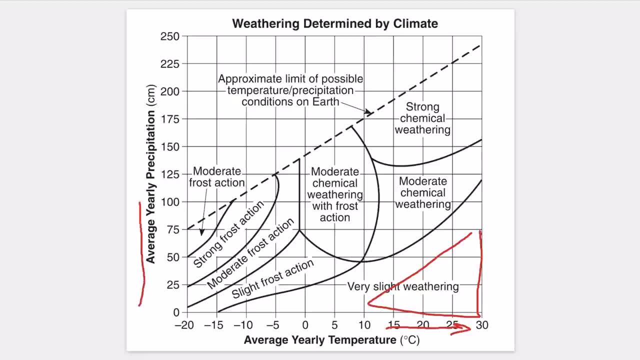 but not a lot of moisture Because, remember, if we go up on the chart, that's a wetter area. So this is an area right here that's hot and dry. Hot and dry, we don't really see a lot of weathering. We might get some wind abrasion, like in the desert, but nothing too severe. If we then switch up to an area that is higher on the chart that is hotter and wetter, that's where we're going to start to see more of this chemical weathering. This carbonation occurs a lot and a lot faster in areas that are hot and wet. We see a lot of. 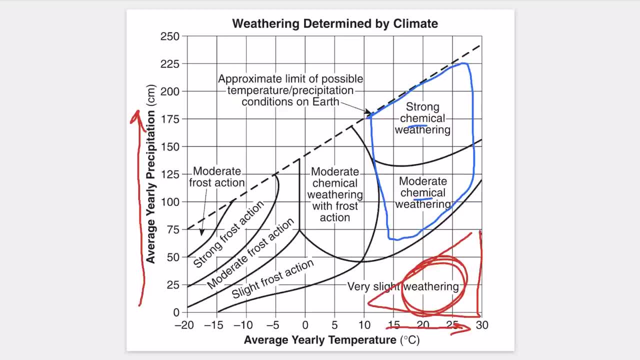 moisture, limestone caves and sinkholes in a place like Florida, for example, where it's very warm and wet. On the other hand, if we go to the left side, where it's colder, lower temperatures, this is where we're going to start to see frost action happening, because this is where we have a lot of change in. 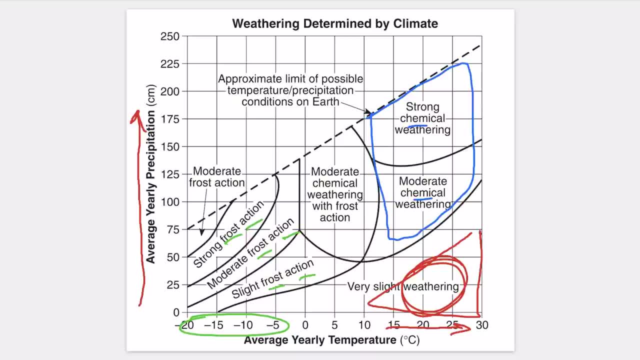 temperature. It's colder, cold enough to get ice and enough water to have the ice forming and melting and forming and melting day after day. Anything up in this top area, up here. these are climate conditions that we don't really see on Earth, so they're not really relevant to what 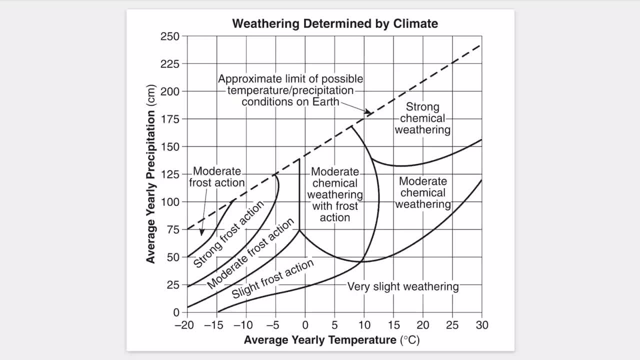 we're talking about. Anyway, this graphic gives you a really good sense of the impact that climate has on the type and the severity of weathering that happens in a particular area. In addition to climate, we also have to look at hardness, So of course we know that all rocks are different. 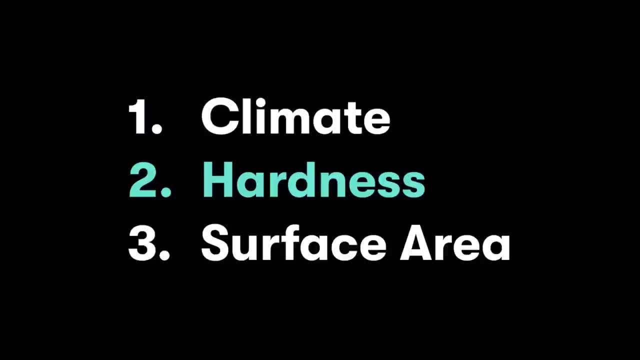 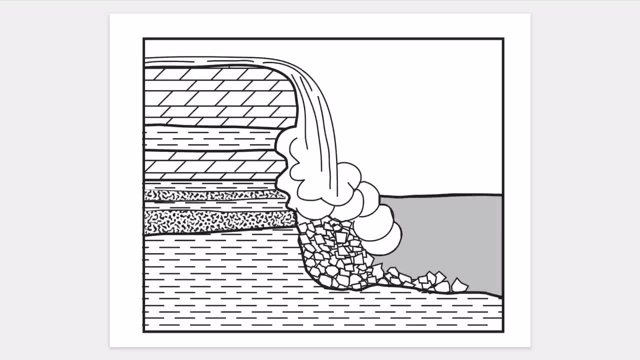 all minerals are different. some are very hard, some are very soft, and that's going to have an impact on how quickly they're going to weather. So if we look at the temperature, we know that the temperature is going to be different from what we're expecting. So if we look at a diagram, 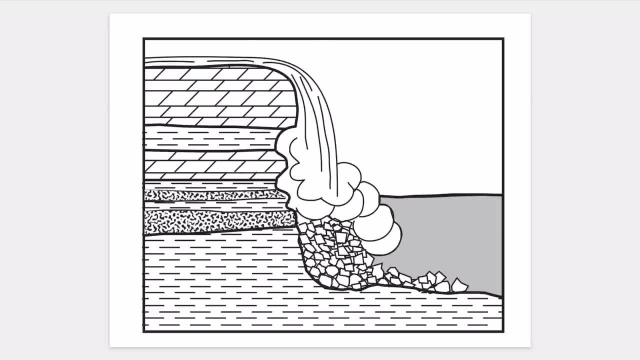 like this, which shows a cross-section of a waterfall. what we'll notice is that some of the rock layers like right in here- right in here, right here- have been worn away more than other rock layers Like this one is not worn away as much these ones down here, this little bit right. 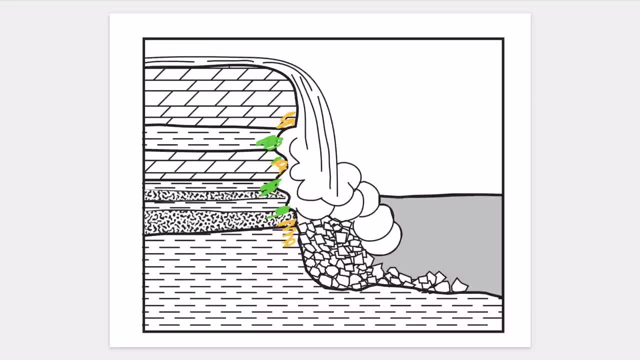 here is not really worn away, And that tells me that these are different types of rock, And so I can conclude that this layer of rock right here, which I believe is like a shale, is a salt, And so this is a softer rock. So when all of this water splashes up on it, it's going to start to wear away. 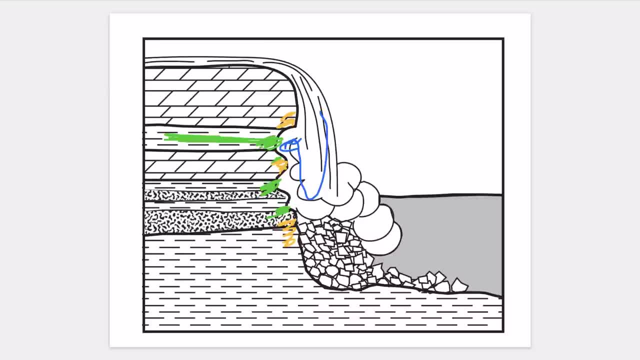 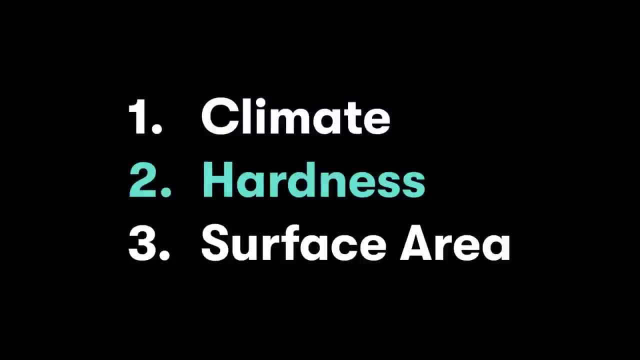 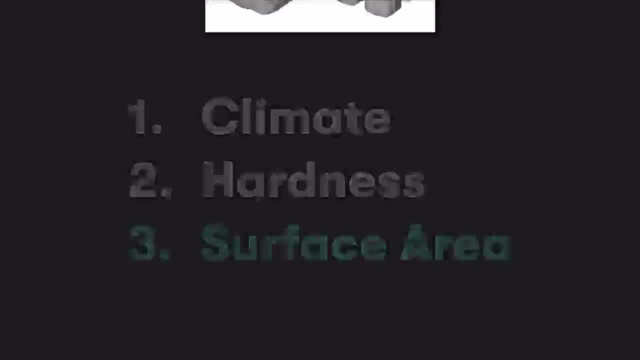 faster than a harder rock like, say, a sandstone. So the hardness of the rock has a big impact on how quickly it's going to be weathered, And so, finally, the last thing we want to look at is surface area. So surface area refers to how much of the rock is actually exposed. So, if I have 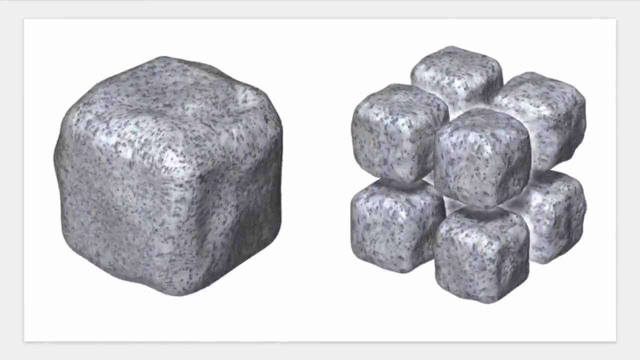 two rocks, like you see here. they're going to be exposed to the elements at a different time, So I'm going to take a different clip, right. So the only part of this rock, for example, that's going to be exposed is the outside of the rock, So the surfaces that I'm highlighting right here. That's. 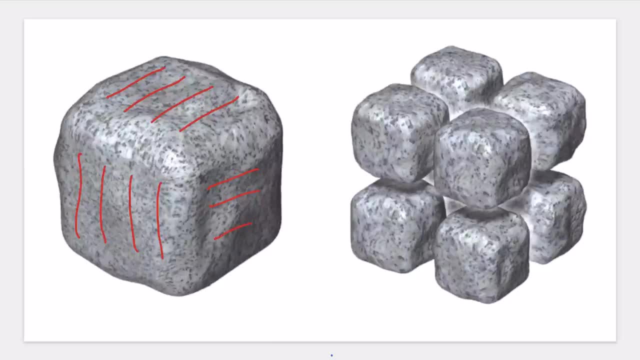 the only part that can get hit by rain and ice and snow and oxygen, et cetera. That's the only part that can be weathered. The center of this rock is not exposed, It's protected And therefore it's not going to be weathered, Whereas in the right-hand side I have the outsides of these rocks. 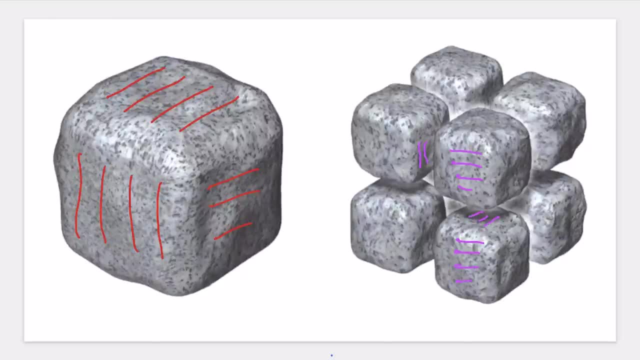 but I also have these inside areas right. So the outside of these rocks is exposed. So, when you right, Because the rock is broken down, we have exposed additional surfaces that can be hit by rain, snow and ice and oxygen and other chemical reactions, And so because this has more surface, 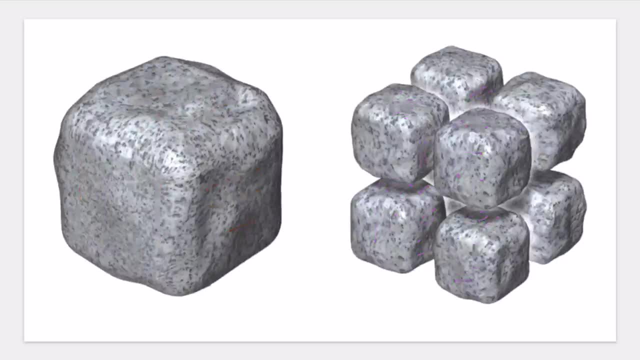 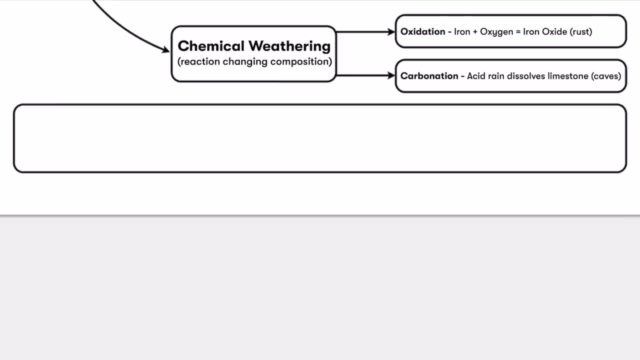 area, the purple, it's going to break down at a faster rate. okay, So we can summarize these three things in our large box at the bottom of the flow chart. We can summarize the factors that are going to affect weathering. okay, So weathering is most affected by these things: the climate, the hardness. 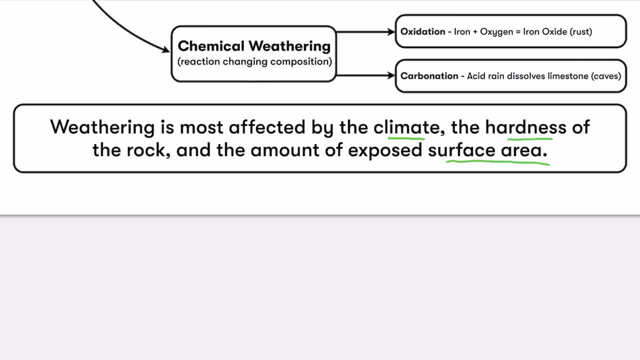 of the rock and the amount of exposed surface area. That's what's really going to dictate how quickly a rock is going to break apart. So in this video we took a look at the different types of weathering, along with some basic definitions of weathering, erosion and deposition, and then 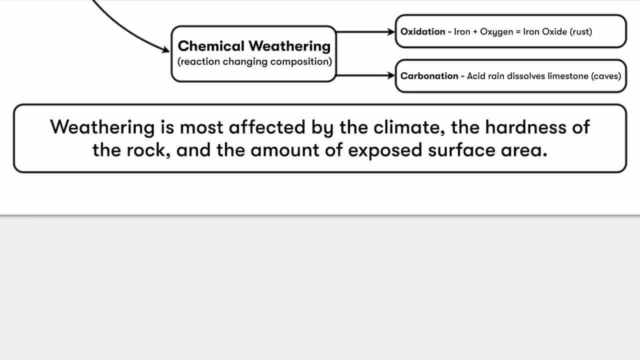 finally at what affects weathering. Shortly I'm going to release another video that's going to go into details about the processes of erosion. Transportation and deposition. are dropping off of sediment, so keep your eye out for those. Thanks for watching.